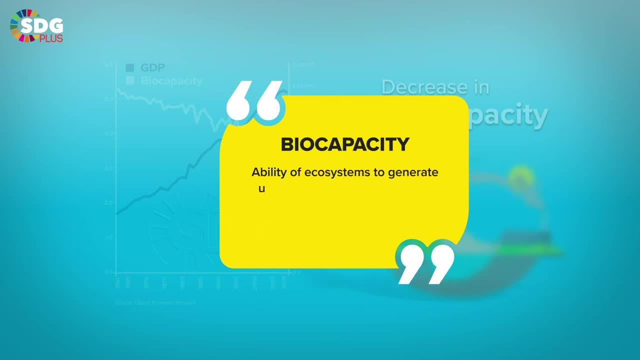 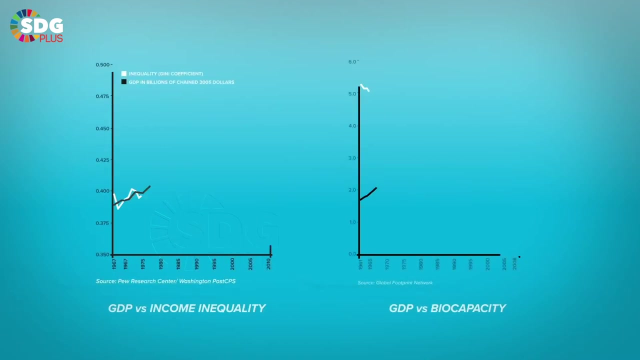 Biocapacity is the ability of ecosystems to generate useful natural resources and to absorb waste materials produced by humans. For example, it is how much oxygen a forest can give us and how much of our CO2 it can absorb. It is evident that GDP does not align with sustainable development. 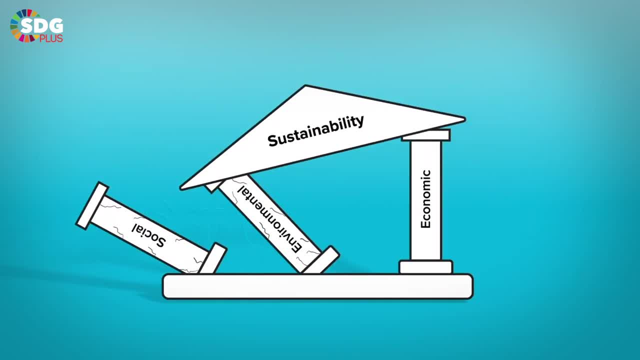 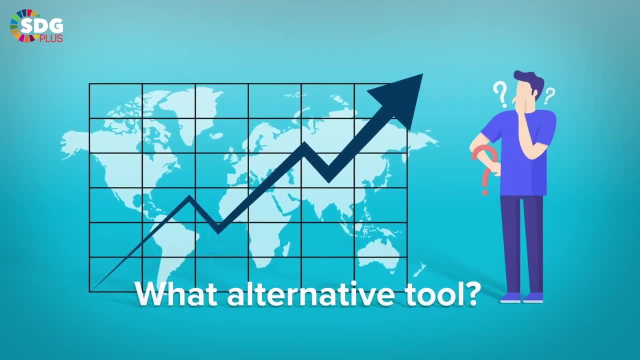 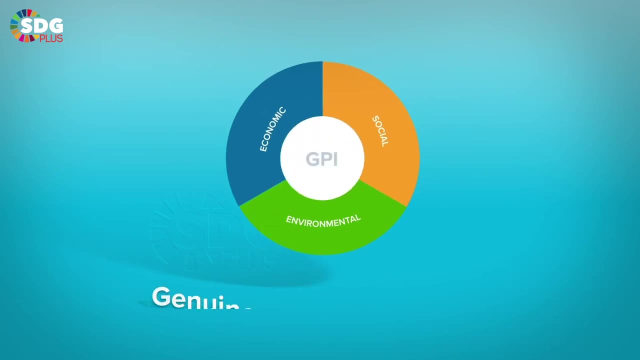 It largely neglects the environmental and social pillars of sustainability. If this old-fashioned approach to global growth is not sustainable, what alternative tool can we use to accurately measure sustainable development? One such assessment tool that has been gaining popularity is the Genuine Progress Indicator. 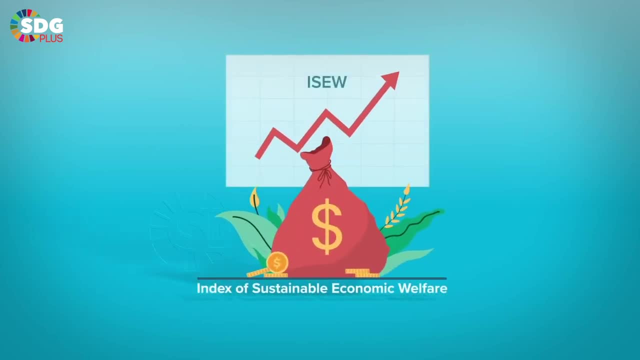 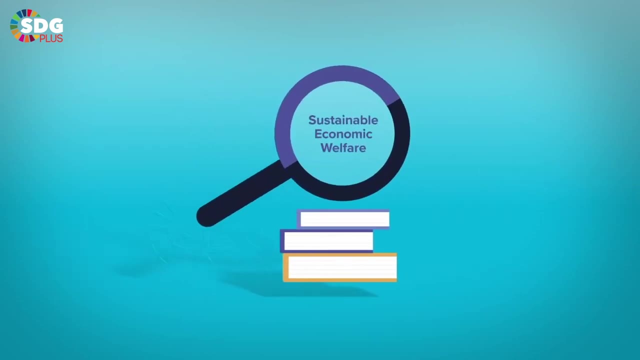 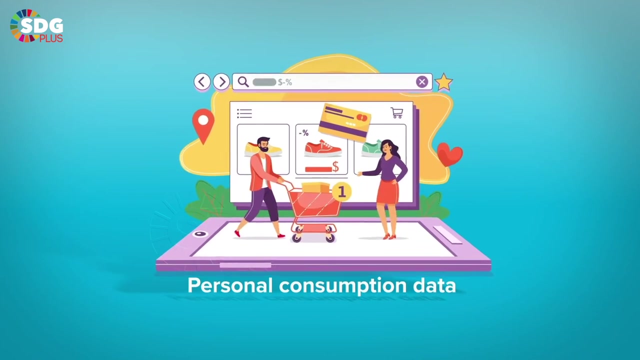 GPI was built on top of the Index of Sustainable Economic Welfare, which was originally proposed by Daly and Cobb in 1989. It was designed to measure sustainable economic welfare and not just financial-focused activities. GPI utilises similar personal consumption data to that of GDP. 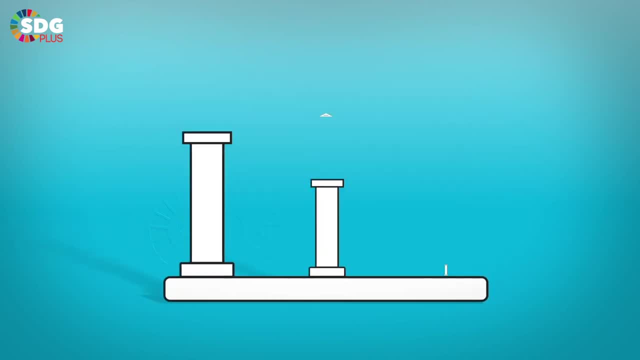 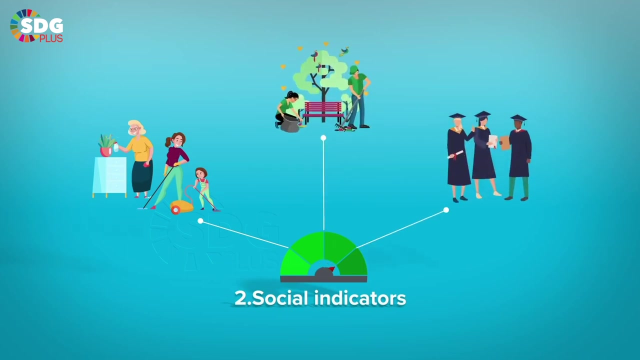 but makes some key changes to how it measures development. It introduces 26 variables that all fall under one of the three pillars of sustainability: Economic indicators that measure income distribution, cost of underemployment and loss of leisure time. Social indicators measure value of household work and parenting, value of volunteer work and value of higher. 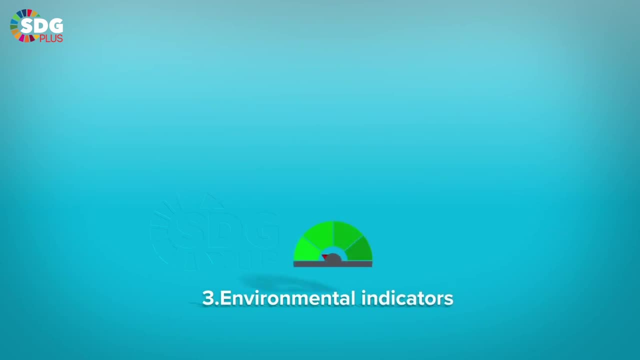 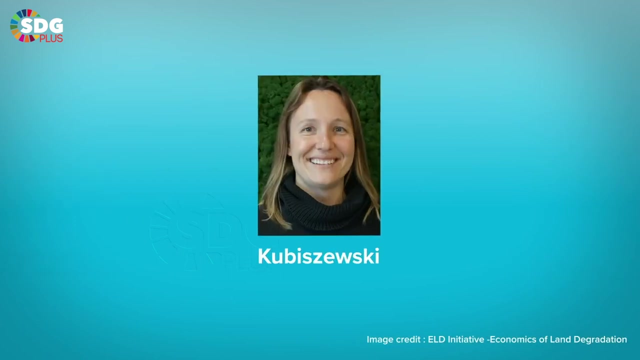 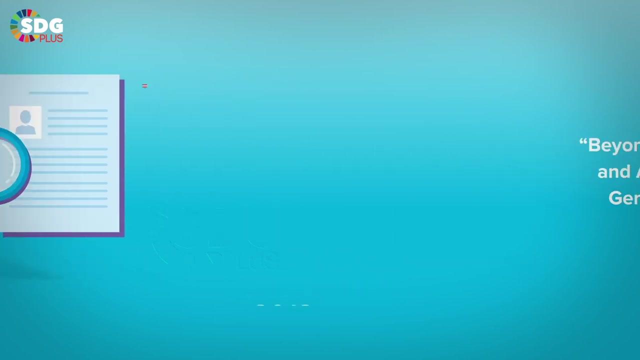 education. environmental indicators that measure cost of water pollution, air pollution, noise pollution, loss of primary forests and damage from carbon emissions. so how bad is gdp at measuring sustainable development? kubizewski, in her 2013 paper beyond gdp measuring and achieving global genuine progress, compared the gdp and gpi progress of 17 countries between 1945 and 1965. gdp and gpi. 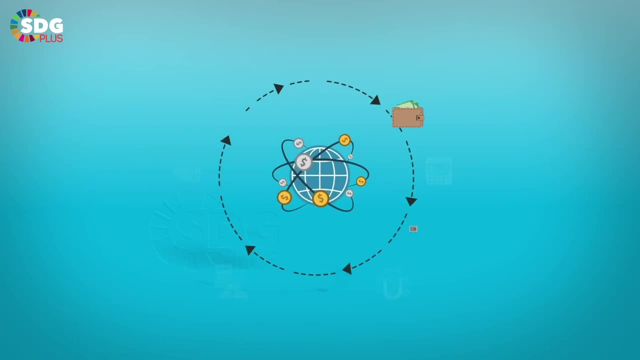 followed a similar growth trajectory in the beginning. it looks like focusing on economic growth seems to bring sustainable development. the likely reason is that if the country gets rich in the future, it will be able to sustain itself and the economy will be able to sustain itself in the future. fewer people are living in poverty. more people have access to education and the 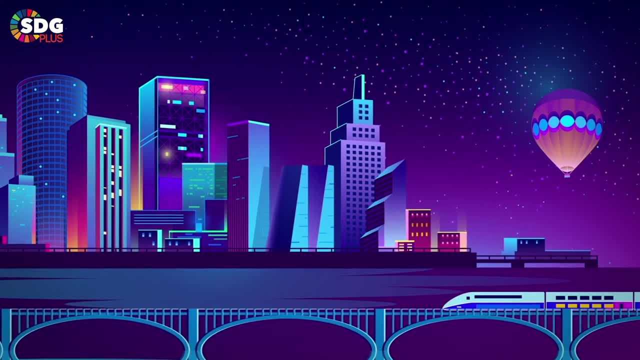 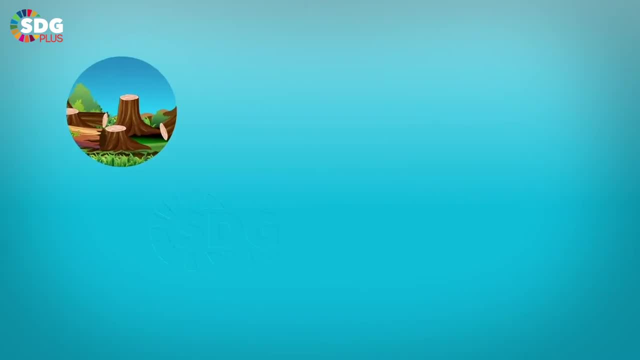 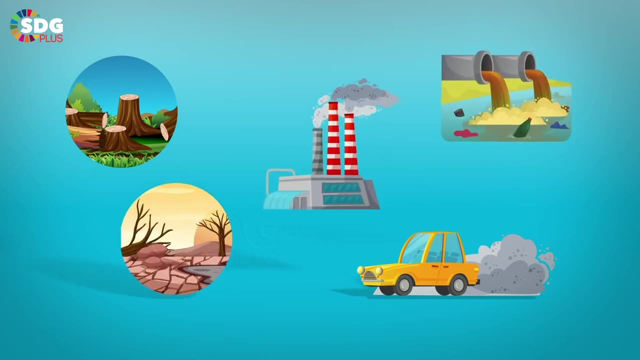 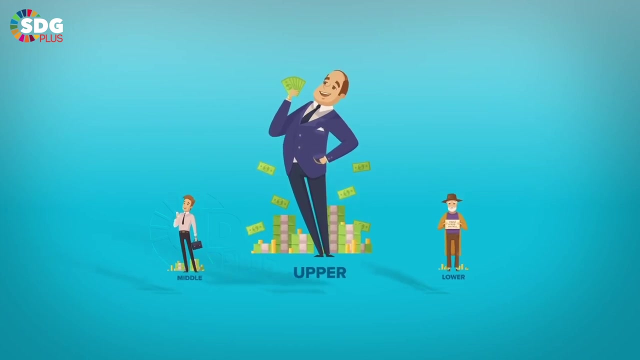 overall infrastructure is more developed. however, this economic honeymoon period ends in the 70s. our rapid industrial growth meant that we were cutting down forests, burning fossil fuels, polluting our soil, air and water at an alarming rate. on top of this, the social gap between the upper, middle and low income household kept widening. 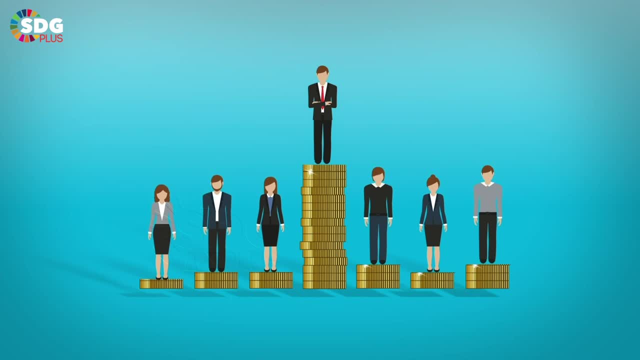 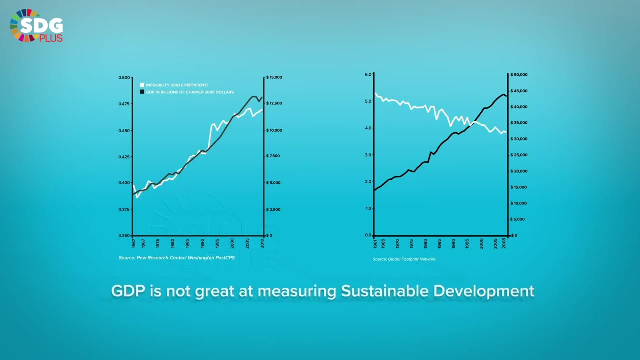 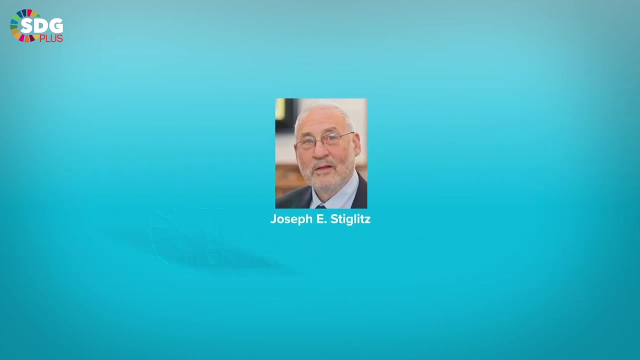 with the rich getting richer and the poor getting poorer, economic growth and sustainable development were drifting apart. we now know that gdp is not great at measuring sustainable development, but why do we need an alternative tool? nobel economist joseph e stiglitz points this out eloquently. 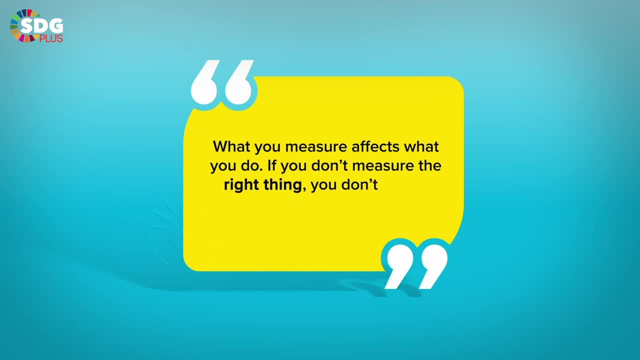 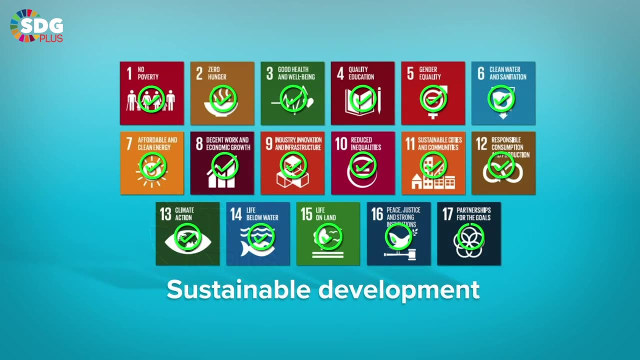 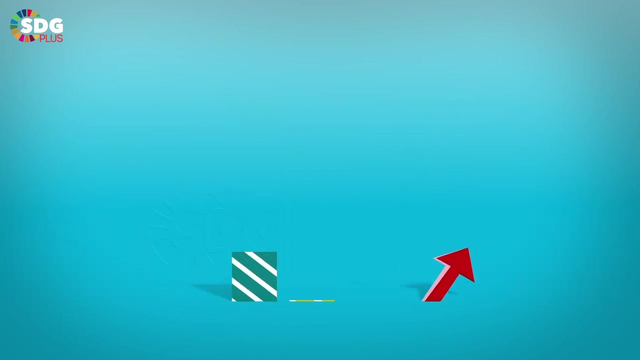 what you measure affects what you do. if you don't measure the right thing, you don't do the right thing. changing how we measure our growth plays a crucial role in the development of our economy. if the world is hoping to achieve a balanced future, our economy needs to move away from maximizing. 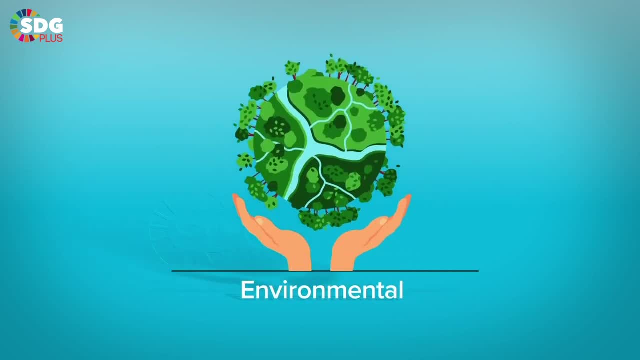 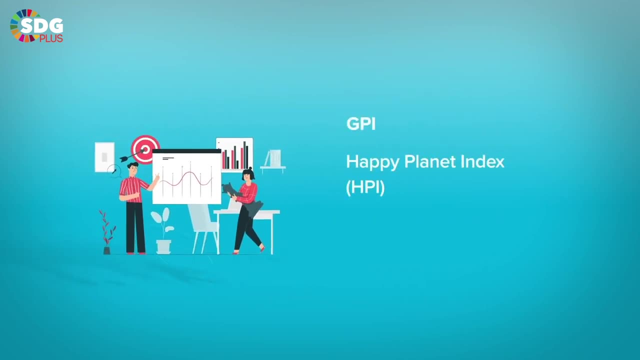 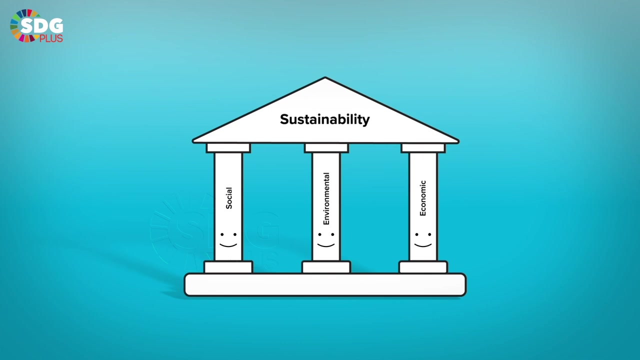 profits and towards social and environmental well-being. in the end, whatever sustainable development metric we adopt, whether it is gpi, happy planet index or human development index- it needs to incorporate variables from all the three pillars of sustainability. here is a quick recap: usa, the country with the highest GDP and the highest GDP in the world, is the country with the highest GDP in the world. 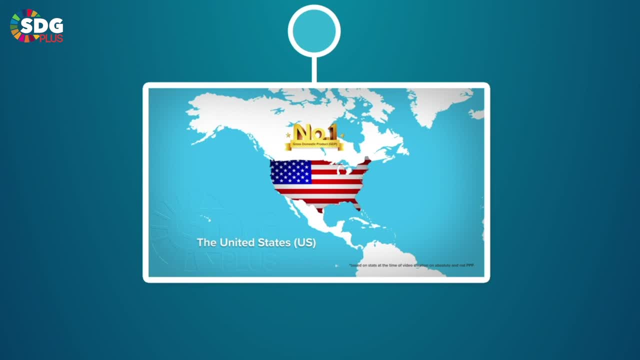 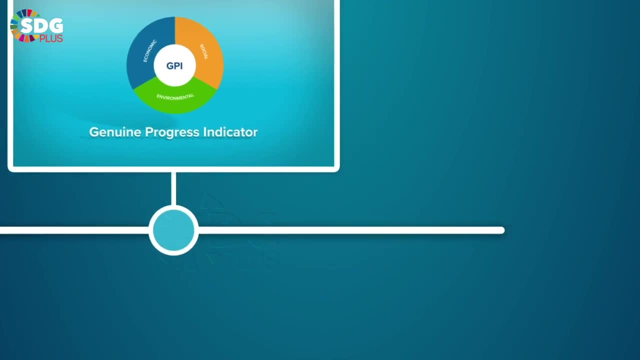 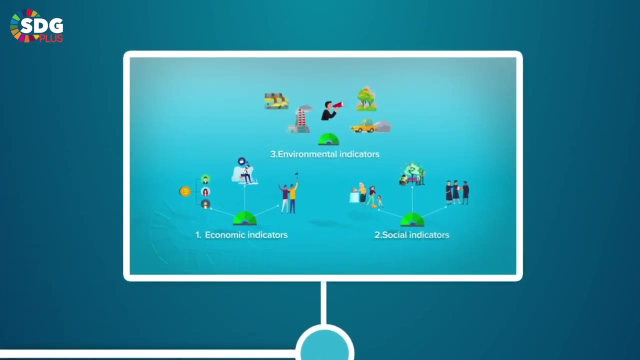 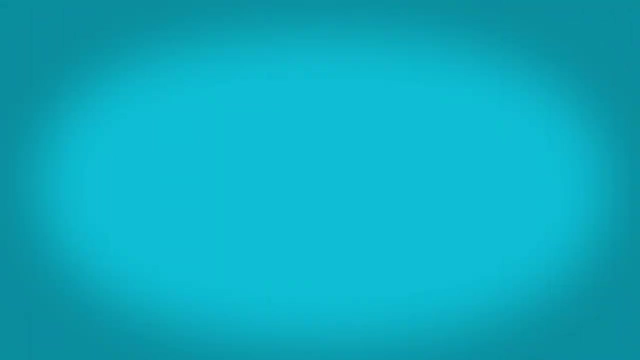 is dealing with rising social and environmental problems. using gpi could be an alternative tool to measure sustainable development. relying on economic growth and GDP is unsustainable in the long run. to achieve sustainable development, we need to change the way we measure growth. thanks for watching. hope you enjoyed our video. if you did, leave us a like and subscribe to our channel. 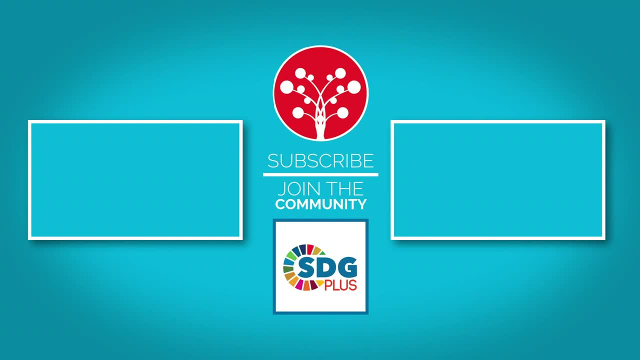 if you did leave us a like and subscribe to our channel. if you did leave us a like and subscribe to our channel, if you haven't already, and let us know in the comments what you'd like us to cover next. if you'd like to learn more about sustainability and test your knowledge, go to our website.